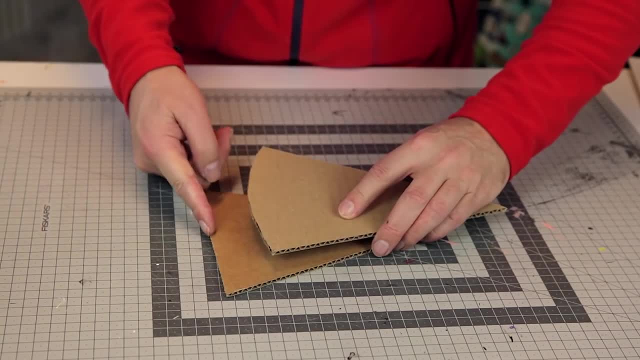 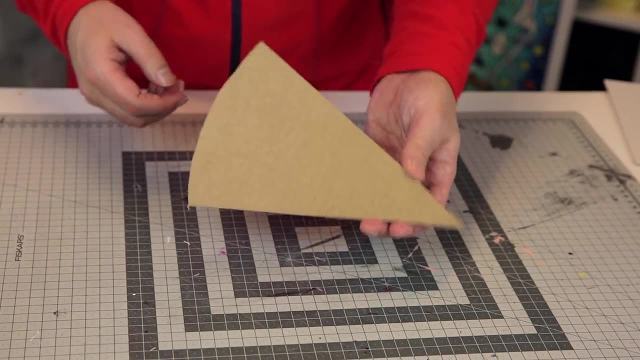 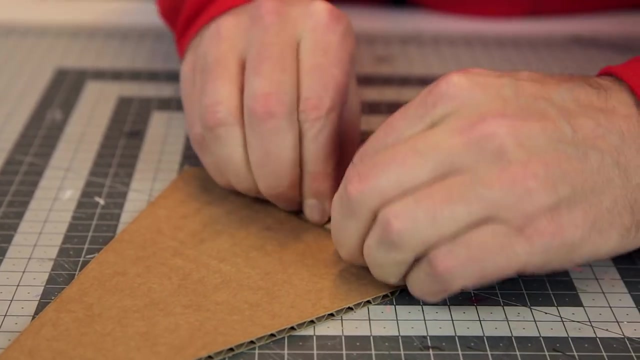 shape, And then you cut along here to make a nice curve like I have here. So this is our starting point for the pizza slice. Next we start folding the curved edge. So we fold a bit, squeeze a bit, fold a bit. 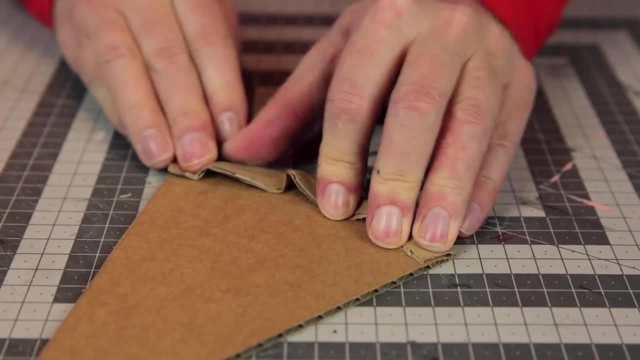 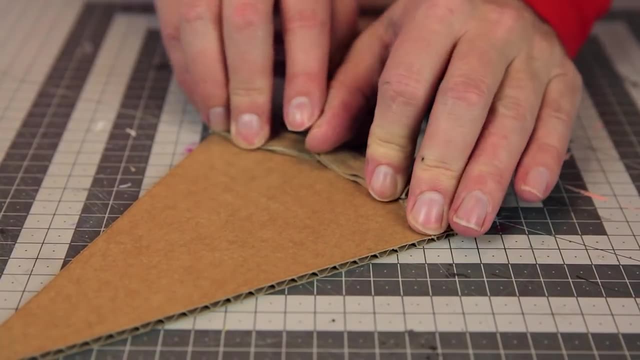 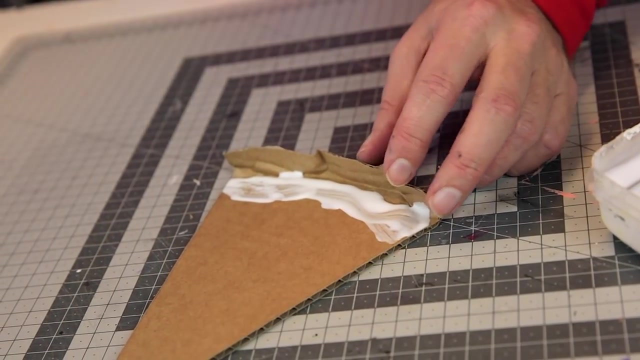 squeeze a bit And then you squash it down like this, just like you would if this was real pizza dough- Then you need some glue. So you take the glue, quite a generous amount of glue along the edge, And then you use some paper clips or some clothing pegs or whatever you have. 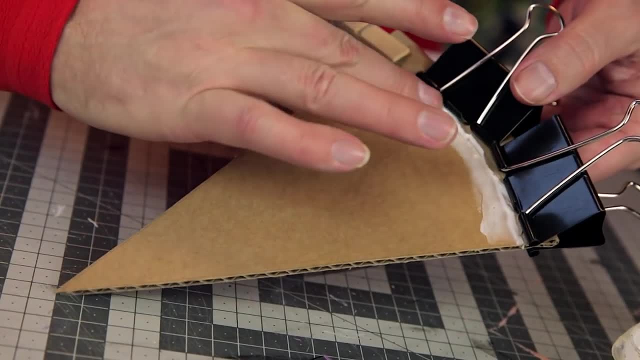 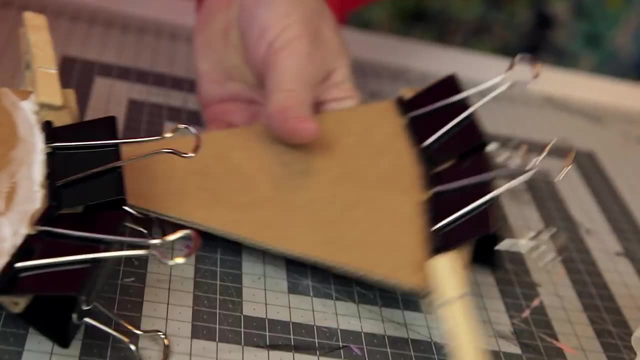 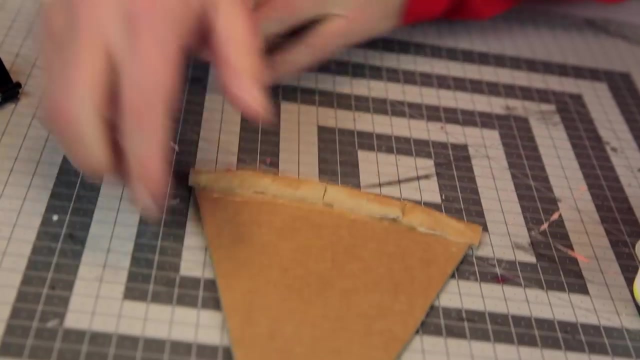 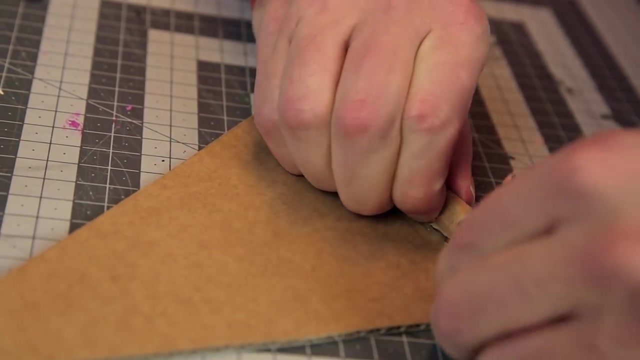 to push this down until it dries. You can wipe away the excess glue if you like. So now this needs to dry, And when it is dry it will look like this: And when we take this off There, you see it's all gone totally solid here. Then you take this solid edge and you 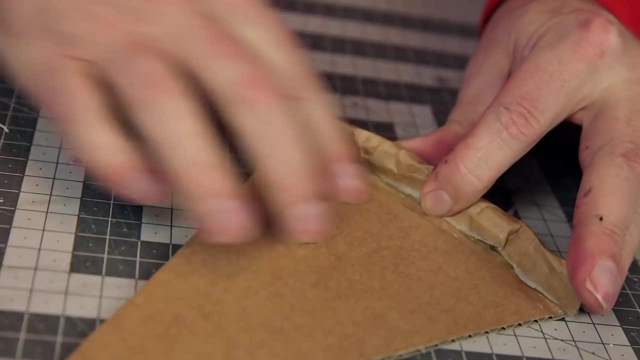 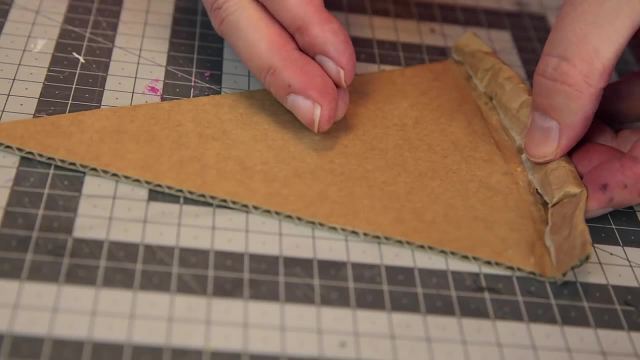 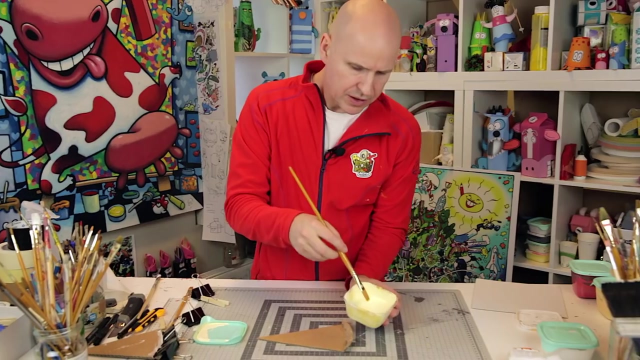 fold it up so that you can put a lot of ingredients in the middle of your pizza slice. Just like that, Just like a nice container there. Okay, so now we are ready to paint Brush. We start with this very, very light yellow. 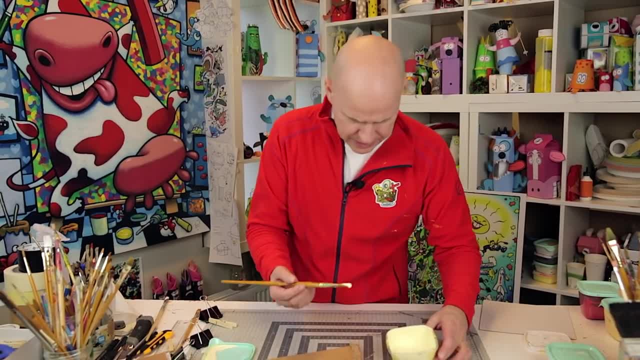 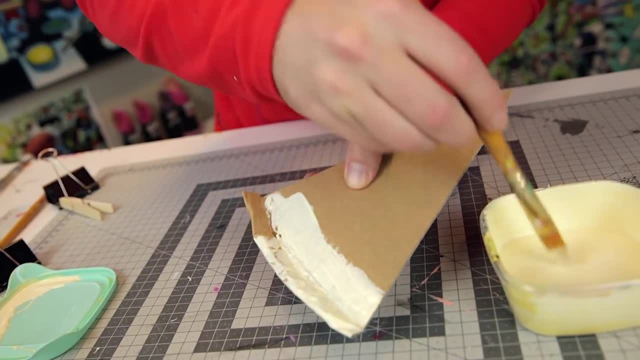 In fact this sort of Half between white and yellow. It's very, very white sort of yellow And we put that on the edge. Going in about this much, Not too long, Don't have to go in too long, And 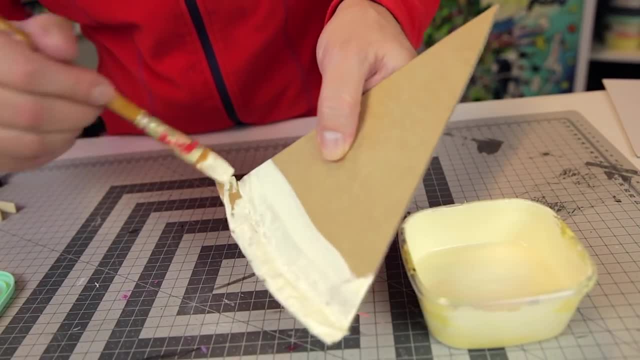 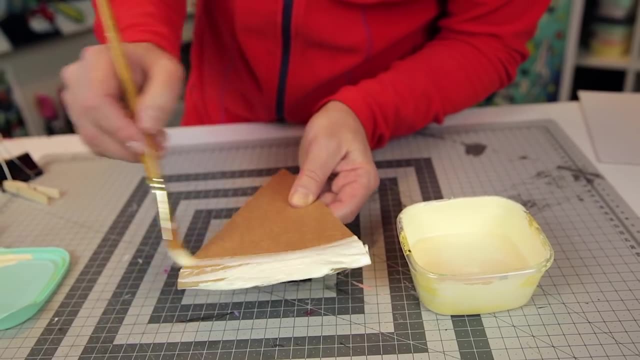 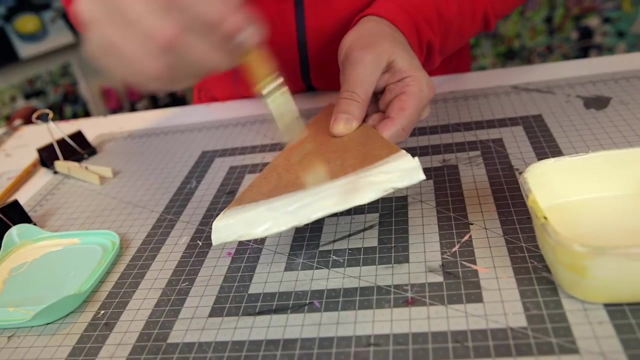 then make sure you get the paint in the little cracks there And go around on the other side a bit too. Don't have to do it too much About this. much Should be just nice. That is going to look gorgeous. So you see, there and there. 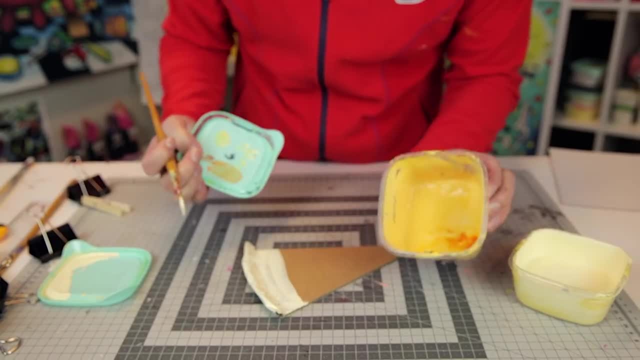 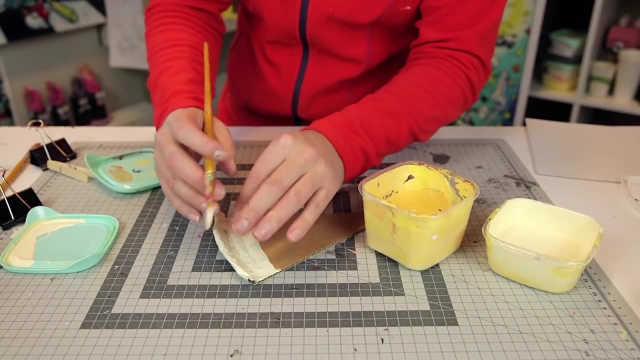 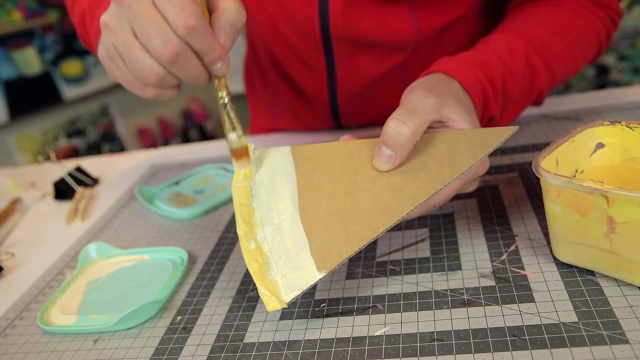 When it is dry. I'm going to use a slightly more sort of browny, yellowy, warm brown to crisp up the crust. Still quite light in color. It will dry darker, But just here on the crust. you can go a little bit darker around on the other side as well. So here, 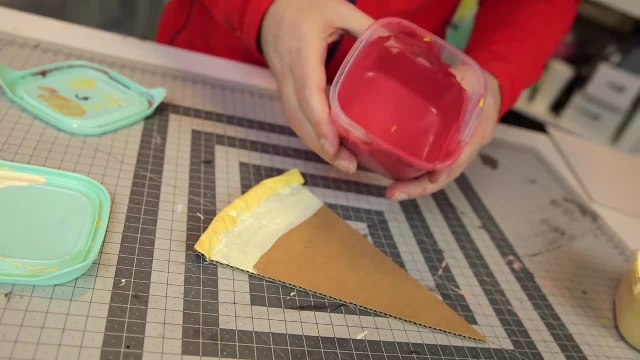 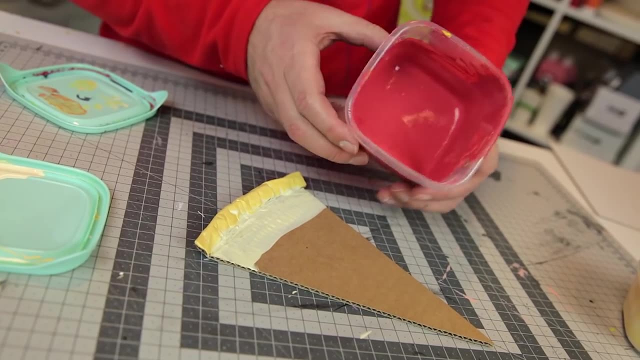 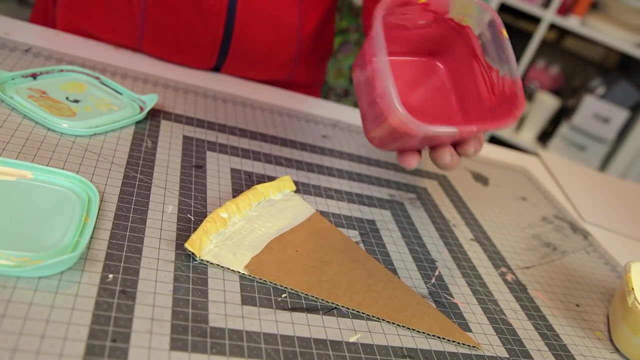 I have the tomatoes Tomato sauce. It's made from red paint And then I mixed in a little bit of yellow, a little bit of white, Just to get it that sort of tomato sauce-like color. And it's kind of thin, So that it reminds us about the consistency of real sauce, So it's easy to pour. So you 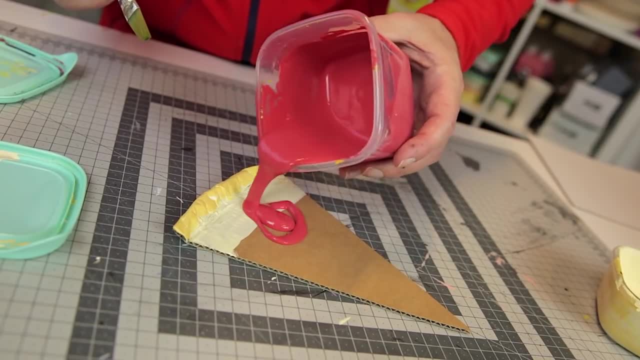 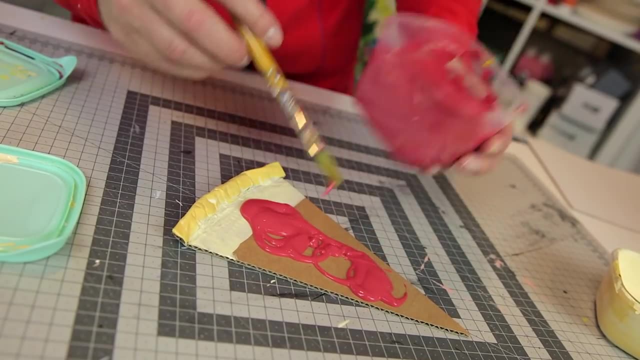 pour this on a bit. Yeah, Look at this Just like you would with the real sauce. Just like that. Not too much, of course, Because then you're going to spill it everywhere, But just pour it on there And then use a. 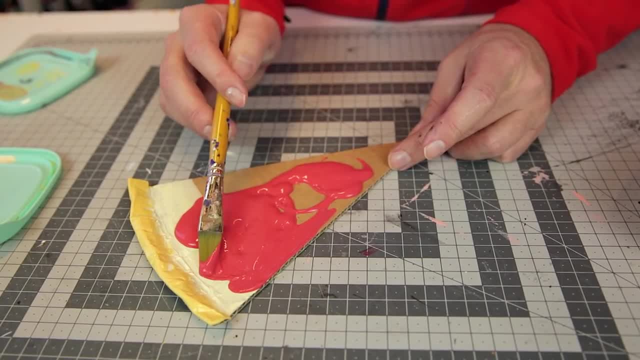 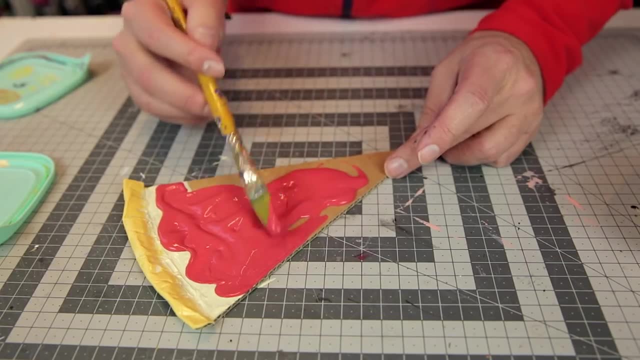 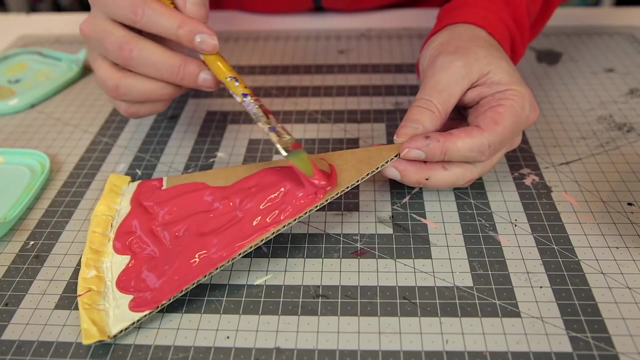 brush to, you know, lay it on. And one thing to remember is that don't go all the way into the edge. Leave a little bit of the lighter color there Makes it look a more authentic Italian, Real Italian pizza, And it's quite thick. This is much more thicker than you. 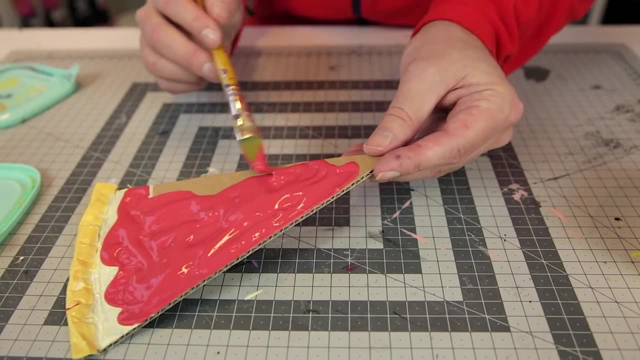 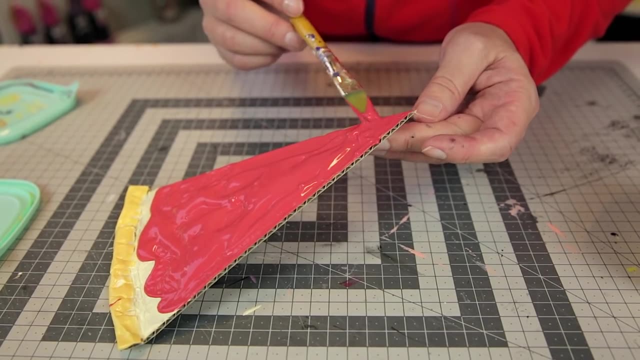 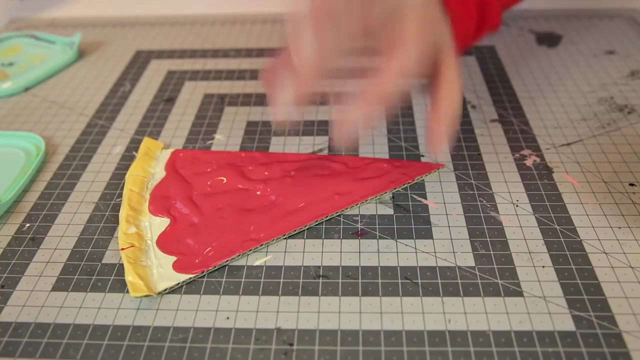 would paint with real paint, I mean as in with normal painting. Now you are copying the feel of real tomato sauce And, by the way, to make the paint flowing like this, I diluted it with quite a bit of water. So into this wet paint you can add: 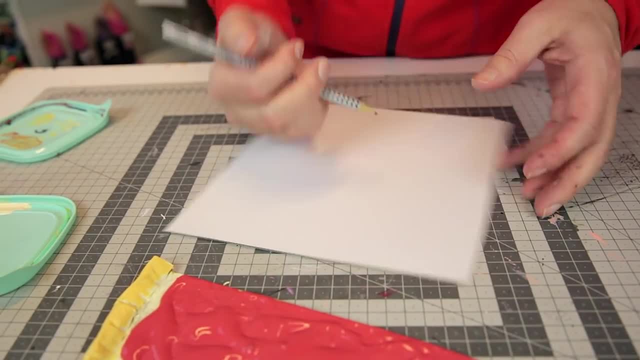 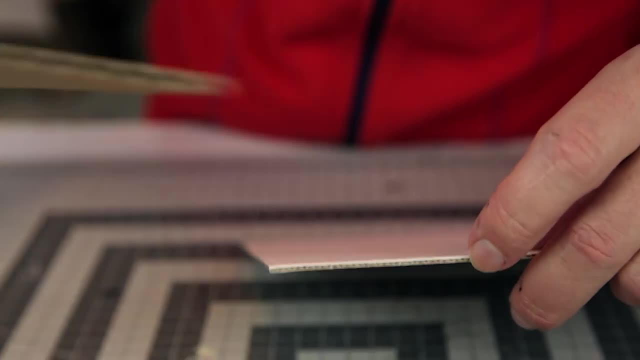 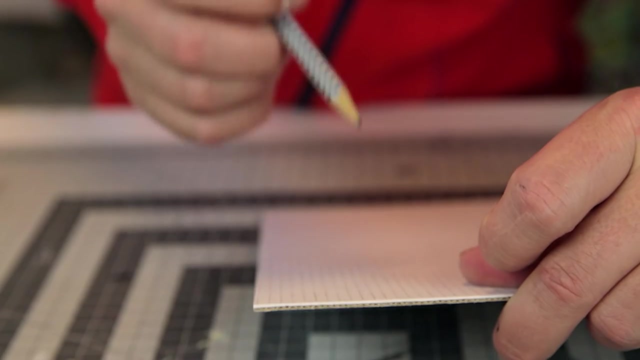 the ingredients. You take a separate piece of cardboard. Look at this cardboard. This cardboard is quite thin. Can you see that? And this cardboard is a bit thicker. Can you see that It's much easier to cut little pieces? You know thick cardboard can be a bit hard to. 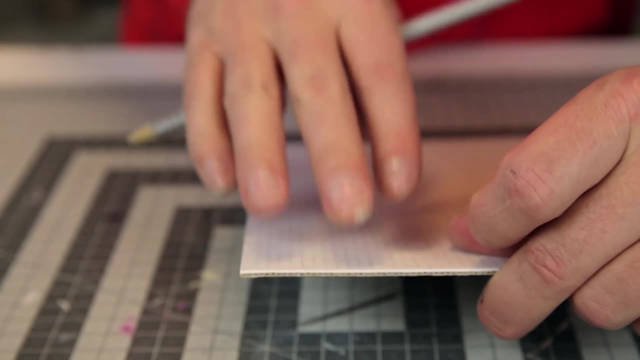 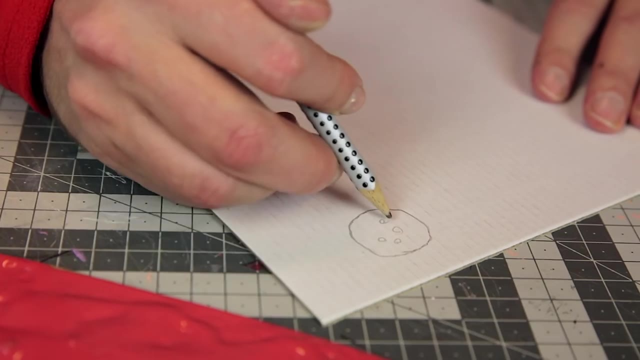 cut corners and stuff. Thin cardboard is better. So find some thin cardboard. It doesn't matter what color, as long as it's thin, Okay, so now we start deciding. Yeah, we would like a bit of cherry tomato pepper cut in. 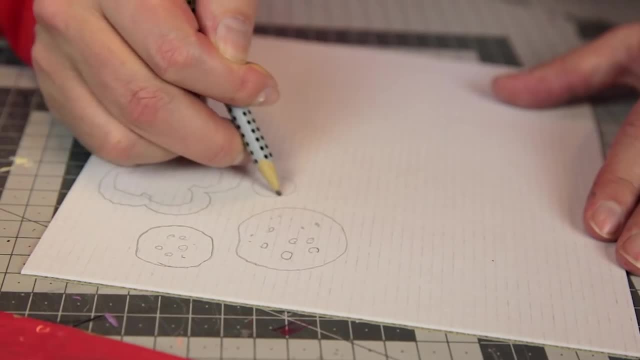 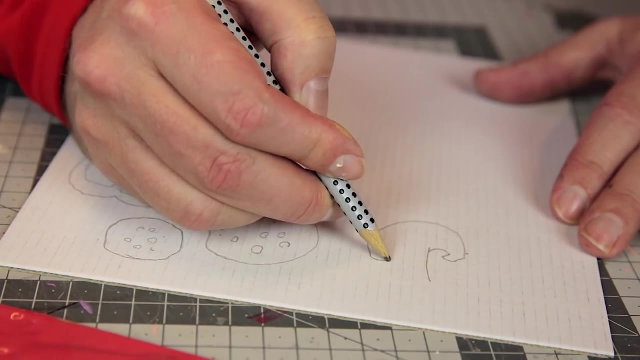 slices pepperoni, some olives perhaps. What else do you want to have? Oh yeah, mushrooms, Mushrooms, Definitely mushrooms. Oh nice, Nice piece of mushroom there, And then you cut them out and paint them. So here I have. 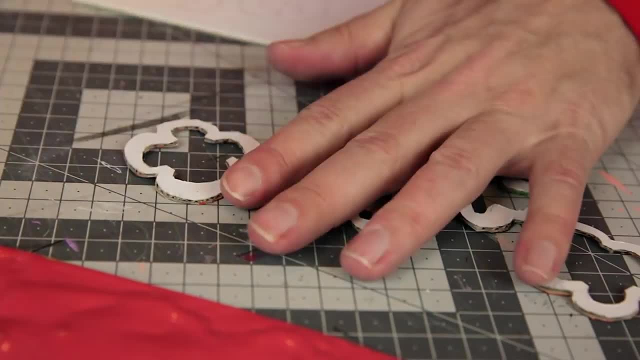 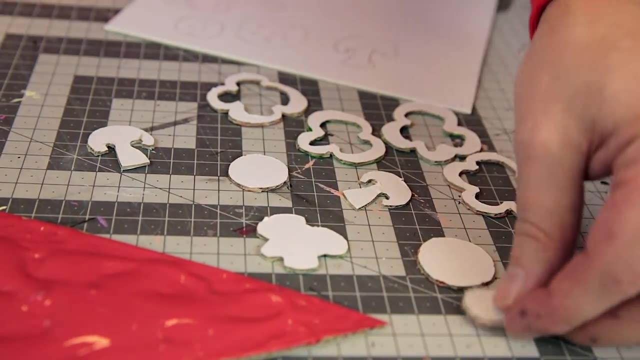 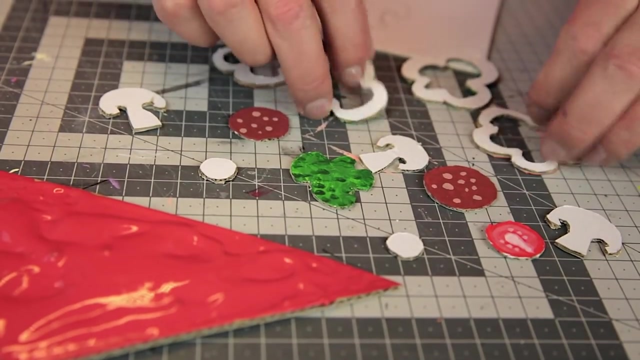 a bunch of pieces that are cut out. These are the peppers, some mushrooms, even a bit of broccoli, pepperoni, mushroom, cherry, tomato and olives. Then I have painted them on the other side. So check this out, Just turn them over and they all got a beautiful painted 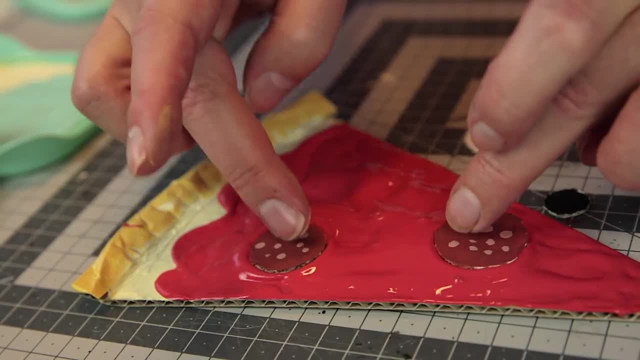 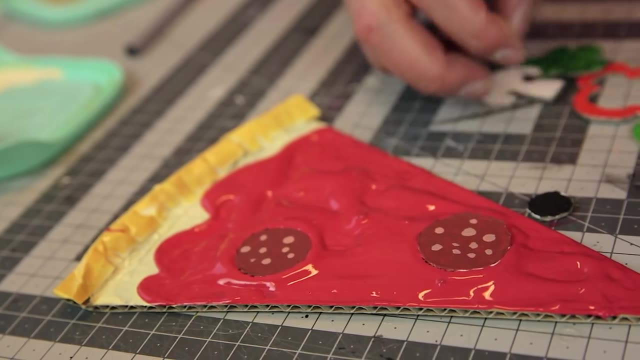 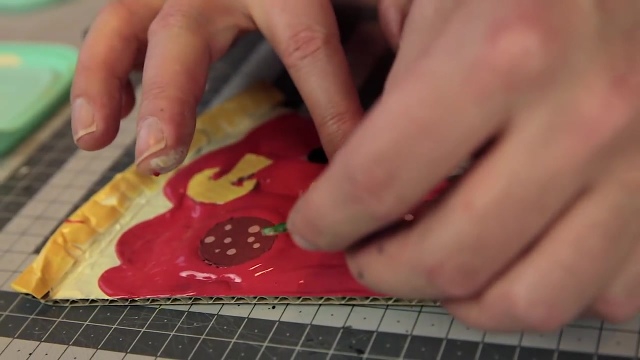 color here. Here we go. Here's pepperoni, Push it in a bit, just like you would with a real pizza. And then, of course, a lot of healthy veggies like mushrooms, cherry, tomato, olive, broccoli. Yeah, I love veggies. by the way, You know, my pizzas are full of veggies, always Okay. 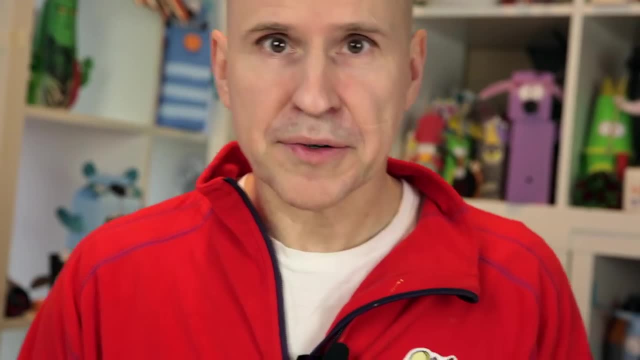 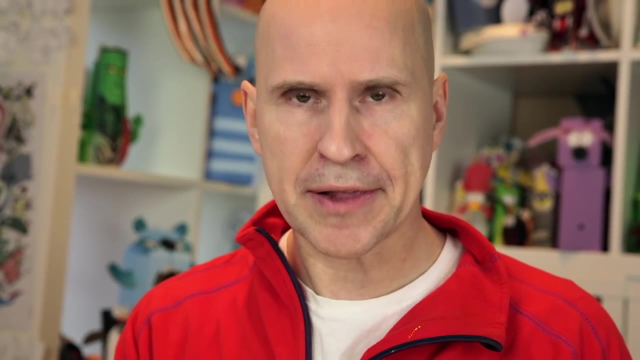 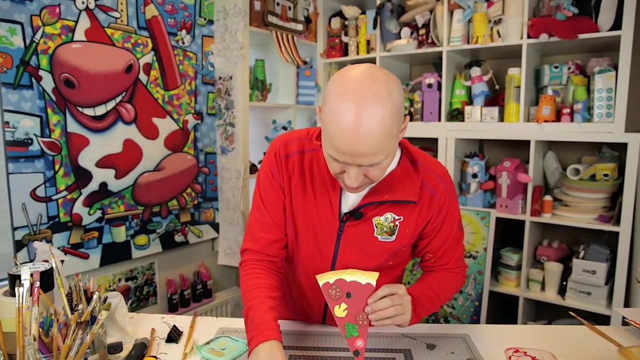 These peppers I'm going to wait with for the second layer. You see, this is just the first layer of ingredients. We are going to add a second layer, but first we need to let it dry And, lucky for us, I have a slice that is already dry, So I can put this aside and continue showing you with 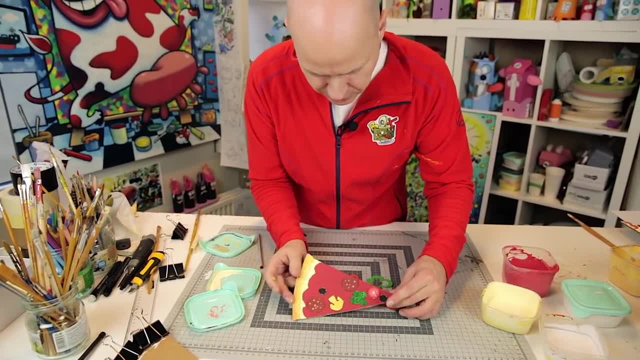 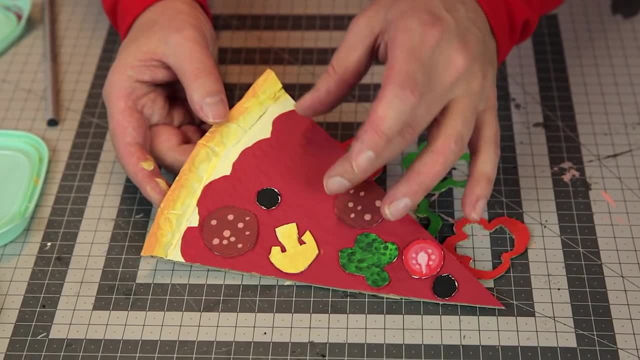 this one. As you can see here, it looks a lot flatter. It's not as voluminous the tomato sauce as we had on the other one, And that's because when the paint dries it will dry flatter. 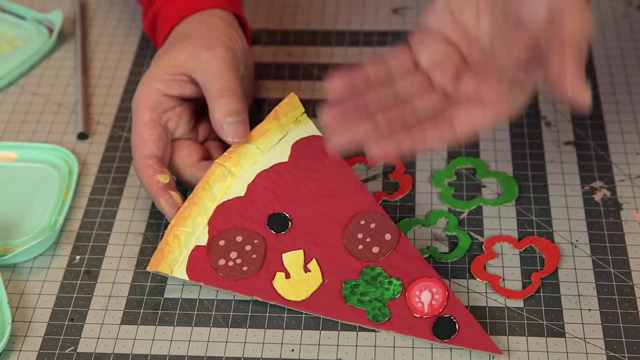 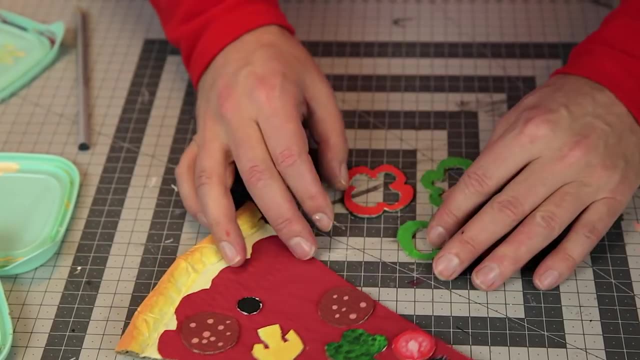 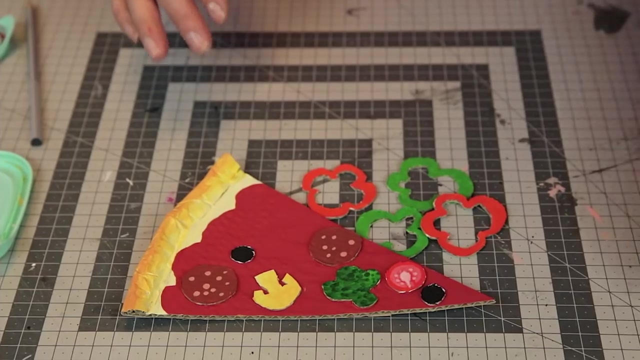 So that's just. you know the way it is, because the water evaporates And you can see, here is an open piece, here- that I didn't add ingredient, but never mind, We have so much to put on, So that's no problem. You see, for the second layer, we need to add the cheese, And here's. 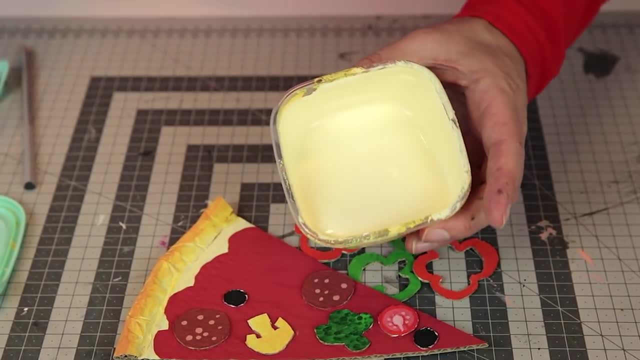 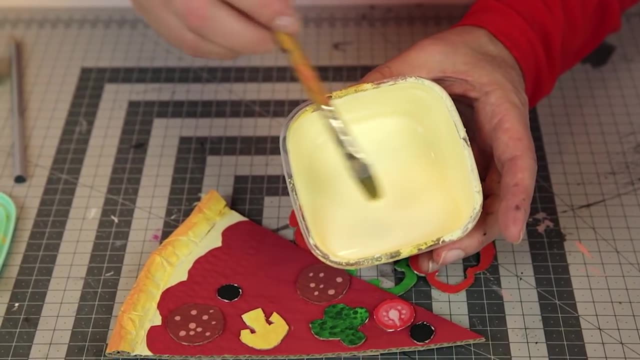 the cheese. Look at that, This is the cheese. So this is a sort of a same color as I used to paint here, Sort of a very white, yellowy white. So I'm going to start with carefully pouring it on where we want it. So I'm going to pour. 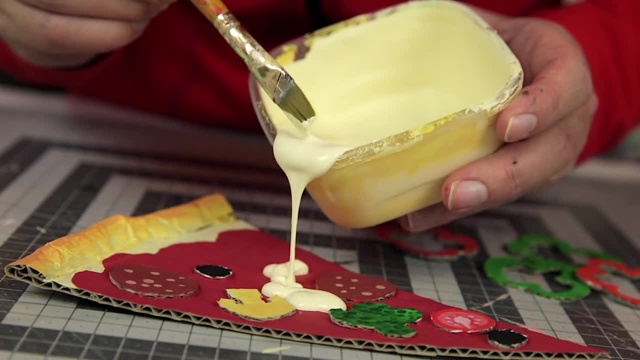 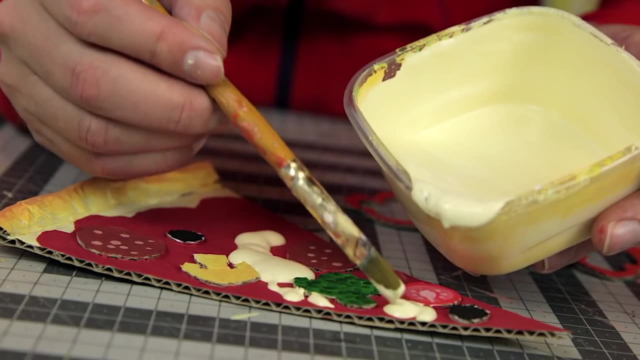 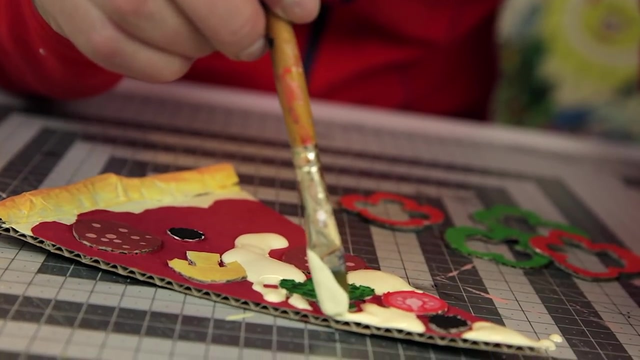 on a little bit in between the ingredients here, particularly when we get to the tip of the pizza slice. You can use the brush if you like to sort of direct the paint. See it sort of flows into the corners in between the ingredients here. 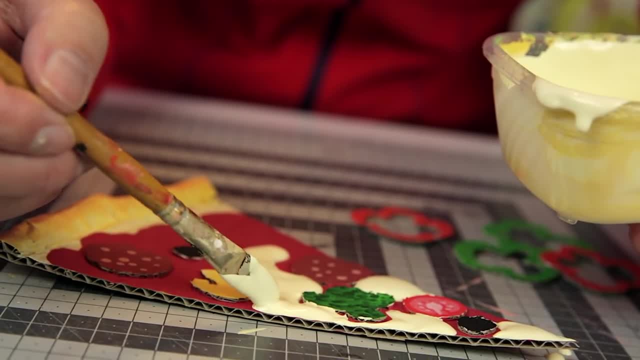 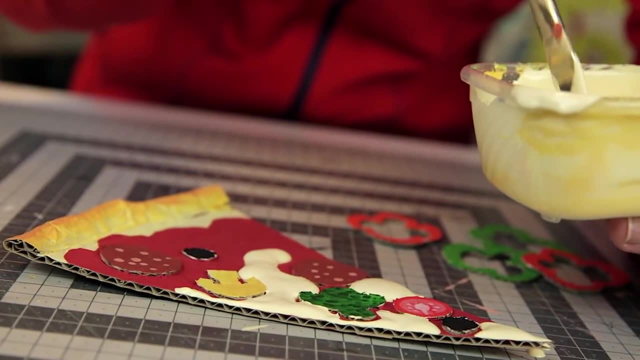 I also suggest that you put a piece of cardboard underneath the pizza and not do it again. You don't want to put it against the cutting board like I do, because it can get quite messy. So how much of the red tomato sauce you want to leave untouched, that's entirely up to. 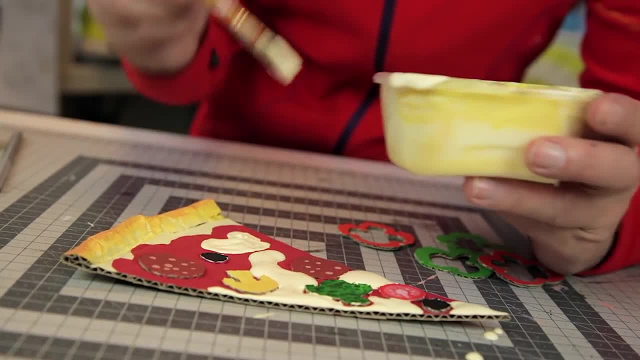 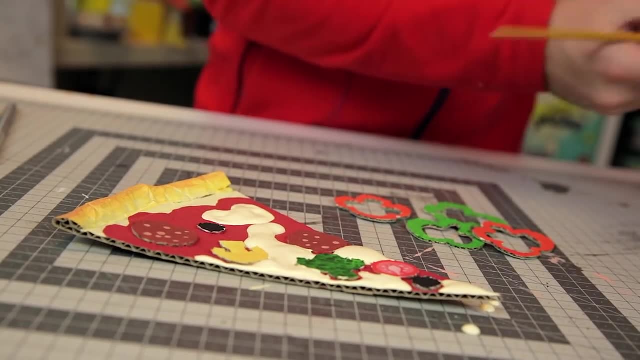 you. So I'm going to just leave some big patches of red untouched, because that looks really good. You don't want to cover up all that delicious tomato sauce. For the next bit of ingredients, I have here red pepper and green pepper. So let's say 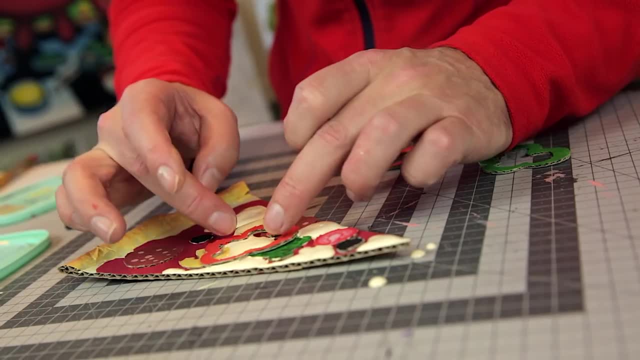 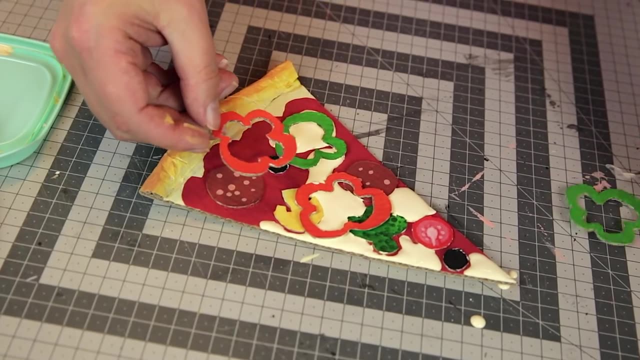 where shall we put it? This is composition here. So I'm going to put a little bit of red pepper and green pepper. So let's say, where shall we put it? This is composition here, folks. maybe here the green one, maybe right here. You can cut them, of course, Maybe. 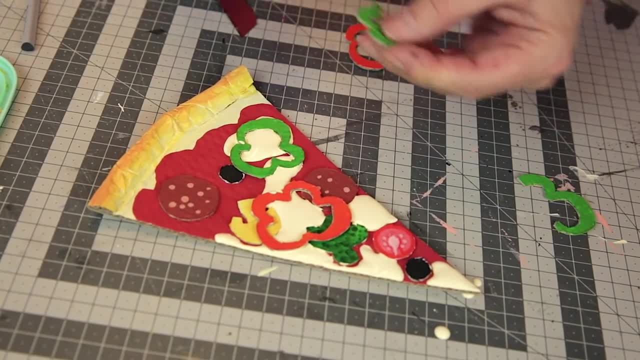 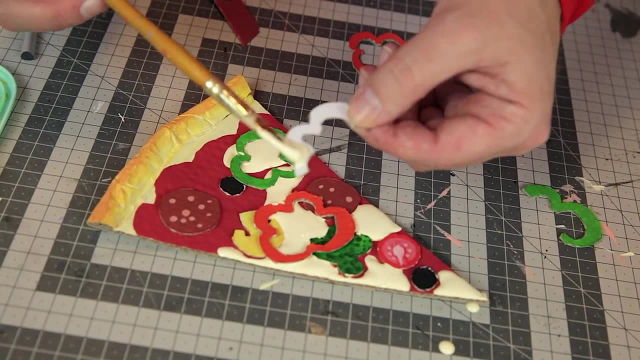 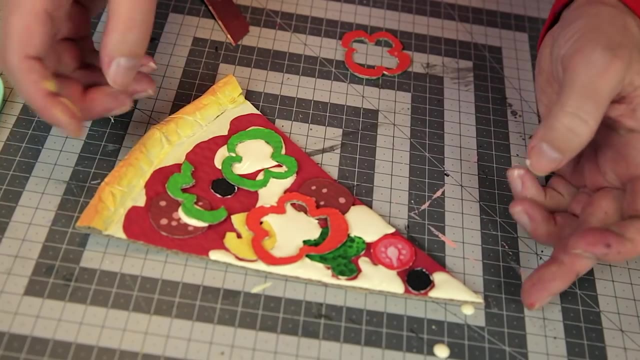 you just like to have half a slice pepper like this. Maybe you want to have it here. In that case, you can just take a little bit of the cheese and then use the cheese as some sort of a glue so that you can glue it on. Oh nice cheese There. now it needs. 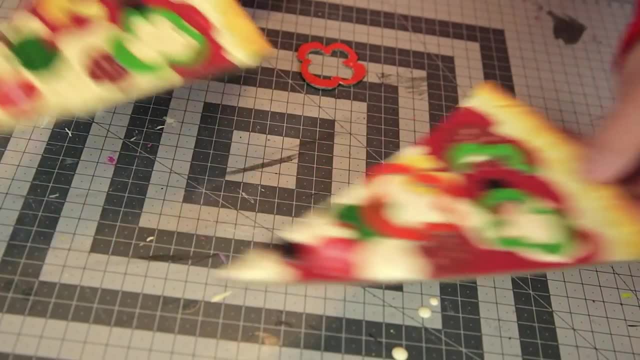 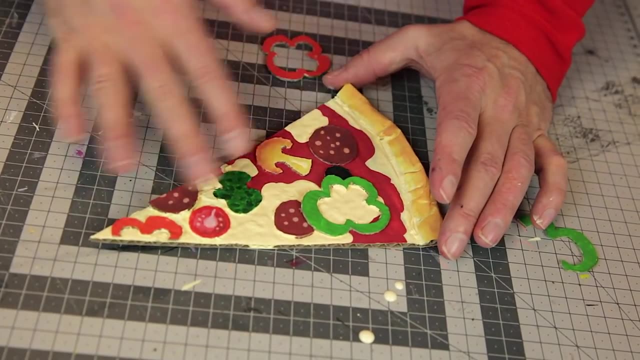 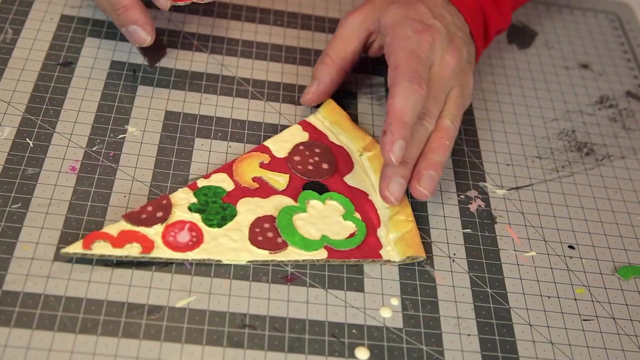 dry and, luckily for me, i have a piece here that is already dry and, as you can see, the cheese doesn't look as much now as it was. that's because it always dries a bit flatter. that's why you can pour on quite a bit, actually, and i'm gonna add the last little bit of um. you know, fine schmecker. 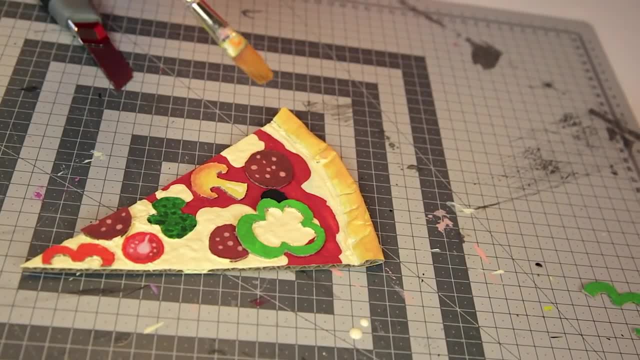 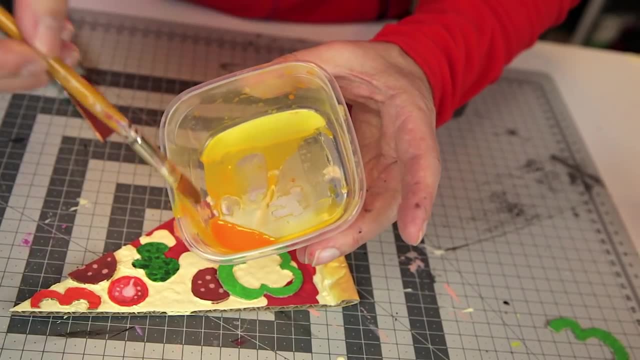 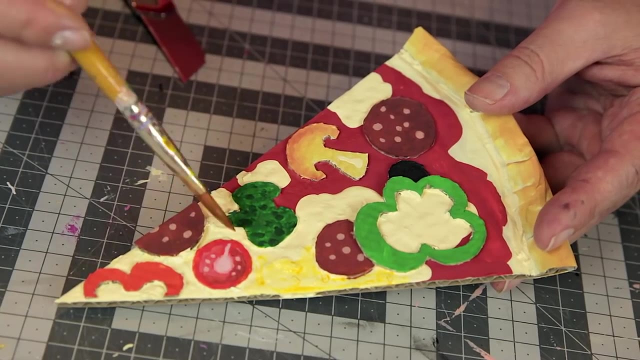 touch to this one. i have a brush here and i have diluted this yellowy orange. this is very yellowy orange, diluted with a lot of water and no white paint in there, so it's transparent. now i'm going to sort of brush on a bit of the warm yellow, because you don't want the cheese to be totally. 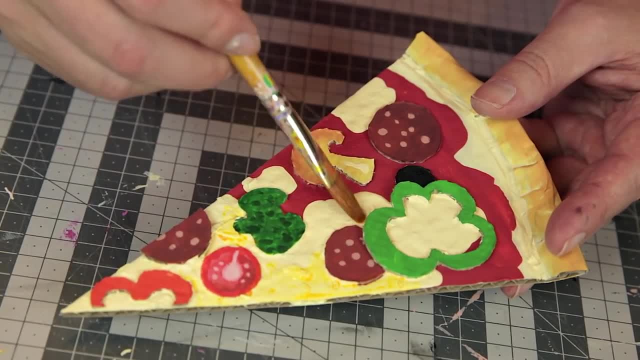 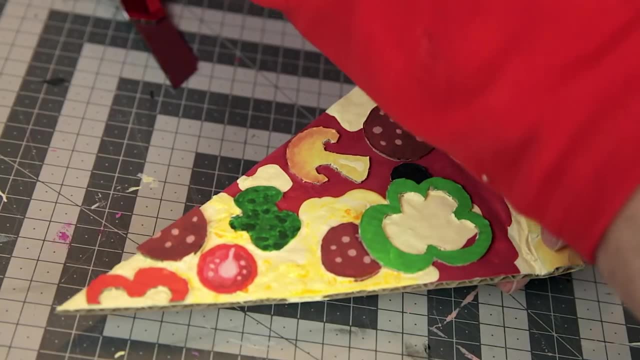 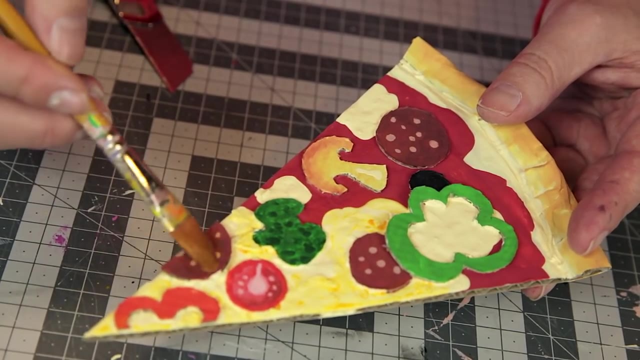 flat in one color. you want it to be a bit sort of mixed between that sort of whiter color and a more warm yellow, so that it copy the look and feel of real cheese and real cheese. you know, once it's baked it can take many different colors. you can also brush this color on here, there and